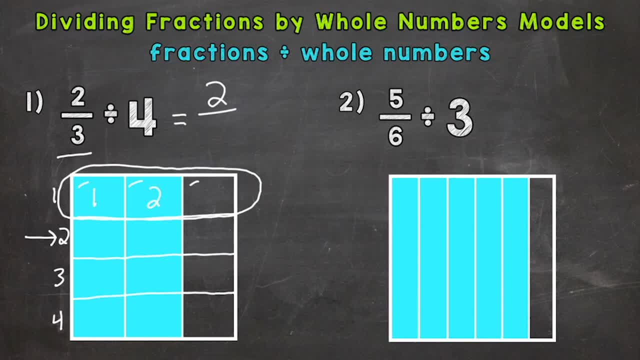 the denominator. So you can do one of two things. The first is just count each one individually, So one, two, three, four, five, six, seven, eight, nine, ten, eleven, twelve, and that will be our denominator, Or we have an array here. so 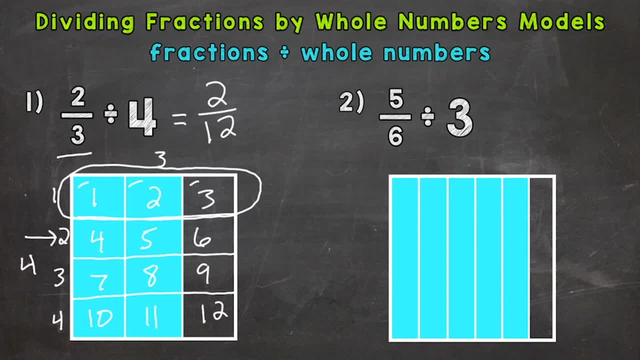 you can do four by three. Four times three gives us that twelve. Either way gives us the same answer of twelve. So our answer is two-twelfths. Now we need to check to see if we can simplify and we can. Two and twelve have a common factor of two. So divide both by two. 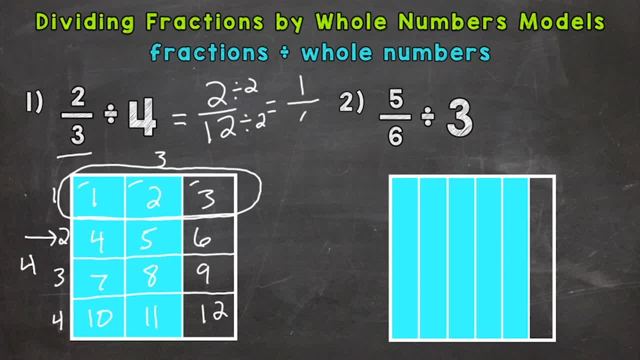 And we get a simplified answer of 1 sixth. So to recap, we started with 2 thirds, split it into 4 equal groups and then we picked one of those groups to see what it equals. It equaled 2 twelfths. then we simplified. 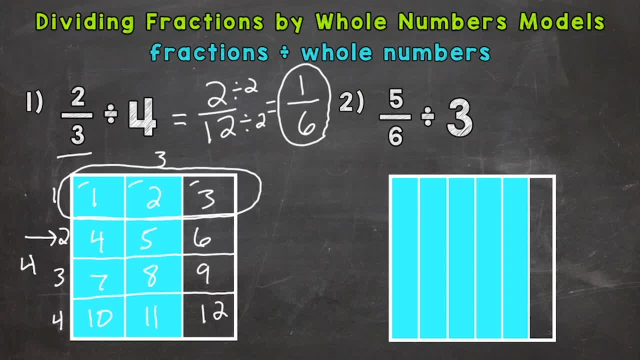 So on to number 2, where we have 5 sixths divided by 3.. So here's our fraction that we start with. Now we need to divide that into 3 equal groups: 1,, 2, and 3. there. 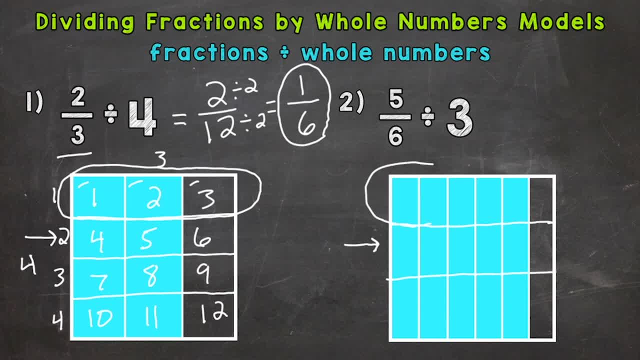 So let's pick one of those equal groups. We'll select the top. Let's see how many pieces are filled in: 1,, 2,, 3,, 4, and 5.. So that is the numerator of our answer. 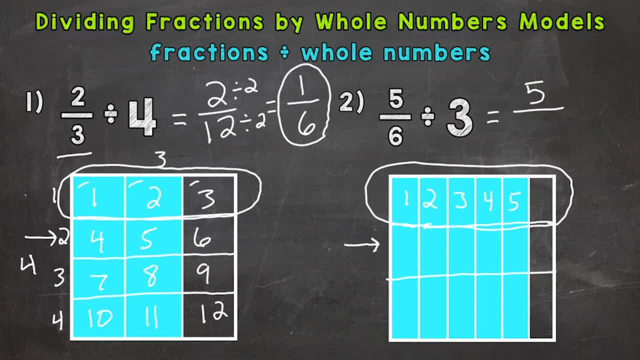 Now we need to see the total pieces in that square. Well, we have a 3 by 6, so 3 times 6. Gives us an answer of 18 total pieces there. Remember, you can do an array and multiply or count them individually. 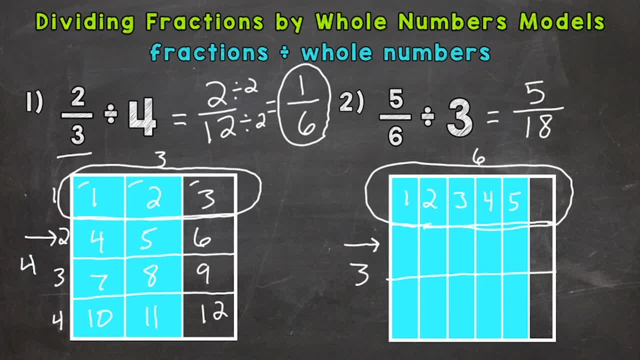 So 5- eighteenths is our answer. Let's see if we can simplify. The only common factor between 5 and 18 is 1.. So this is in simplest form and we are done. The answer is 5- eighteenths. 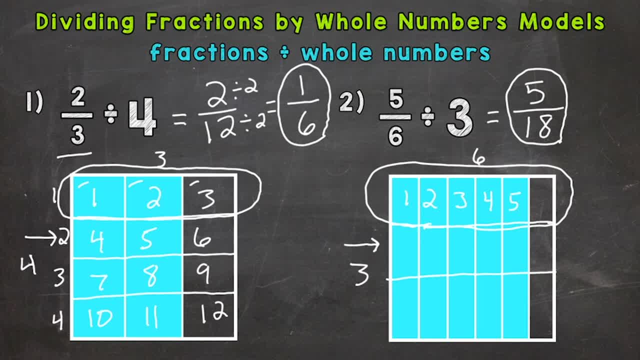 So there you have it. There's how you model dividing fractions by whole numbers. Now I have videos on other situations as far as fractions within division problems, videos that include models and videos that do not include models. So if you're looking for more help with division problems involving fractions,